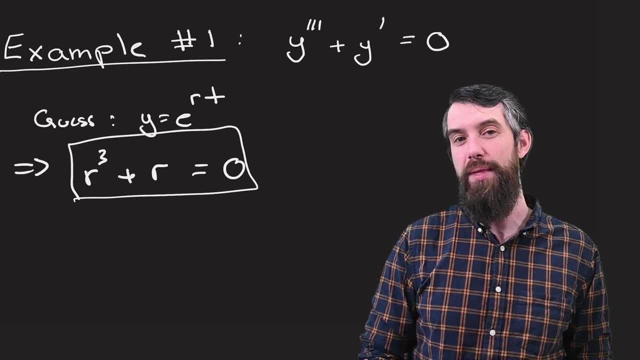 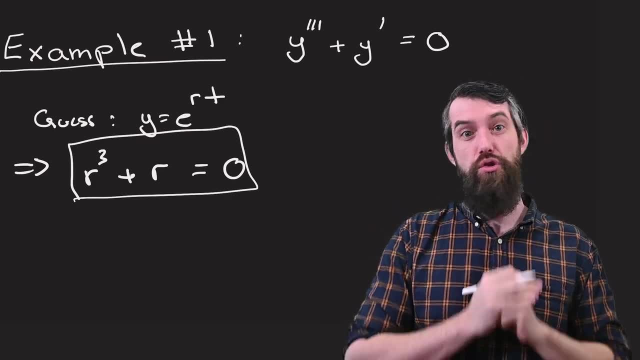 You're just left with this, the so-called characteristic equation. Now, what's relevant here is that this is a polynomial. Now, if you had a degree two polynomial, you can always solve this by the quadratic formula. So any degree two polynomial you could factor. 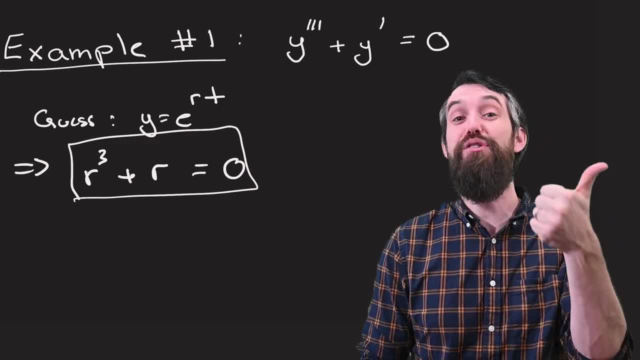 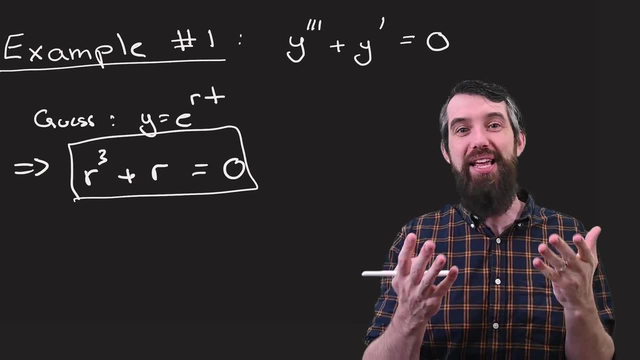 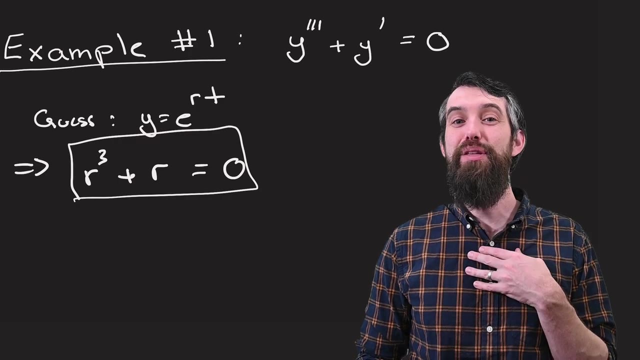 And we've seen that there have been a few different cases. You could have two different real and distinct roots, You could have real repeated roots or you could have a complex pair. So what's going to happen in the third order case? Well, first of all, I can sometimes factor these, but I have to be a little bit more ad hoc about it. 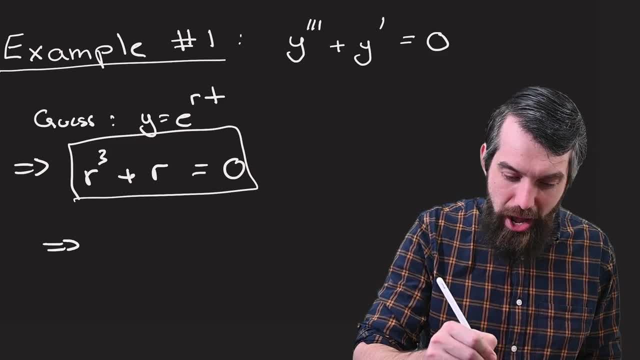 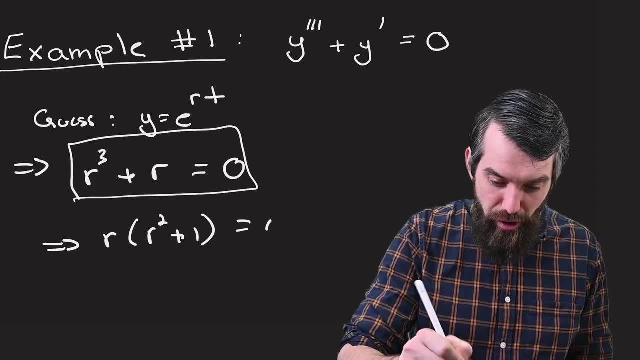 Namely. I'm going to just observe that I could factor out a copy of r and that would leave me with r squared plus one. And then I could do even further if I looked at that r squared plus one. Well, that doesn't factor nicely over the real numbers, but it does over the complex numbers. 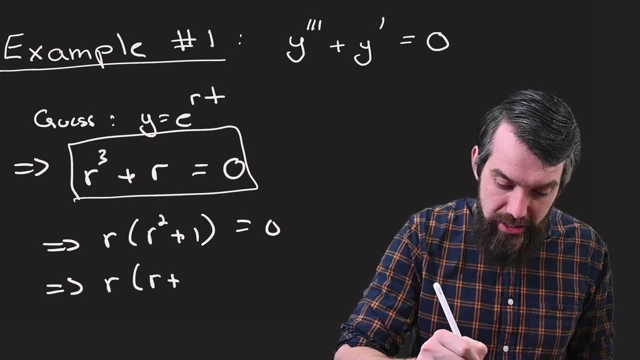 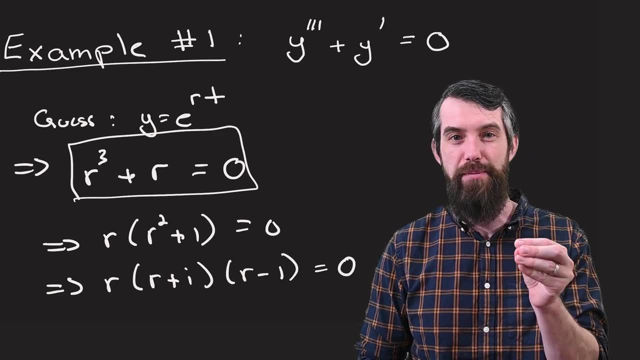 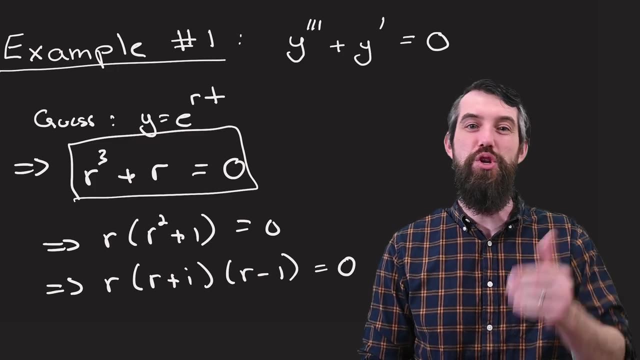 So this could be thought of as r times r plus i and then multiplied by r minus i. I can factor that over the complex numbers or, if you prefer, I could do the quadratic formula on r squared plus one, and that would give me plus or minus i as well, whichever you prefer. 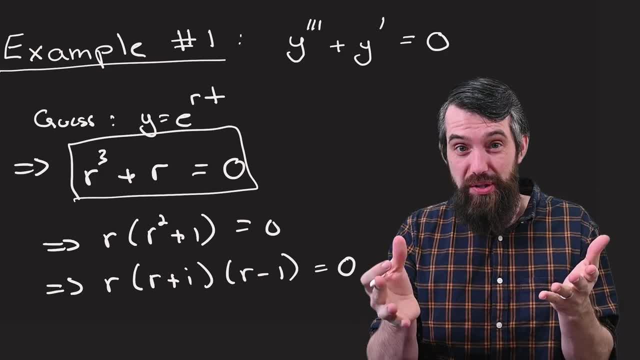 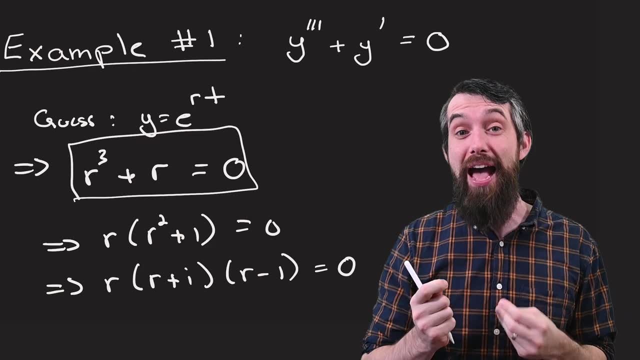 By the way, it's kind of cool for the quadratic formula. We can always solve them. but what about, say, cubic and quartic polynomials? Well, it turns out that you can also always factor a cubic and a quartic polynomial. 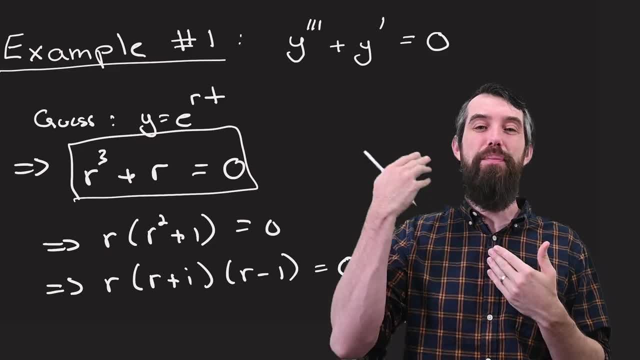 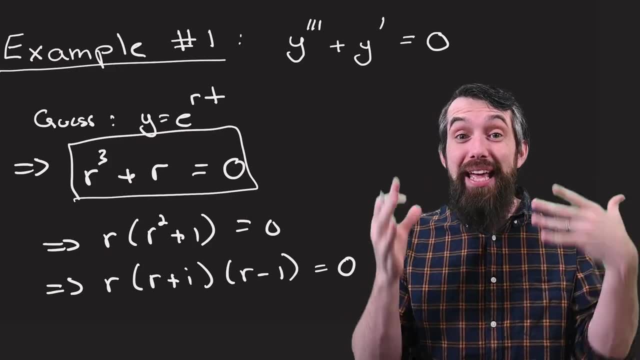 There is an analog of the quadratic formula, but it is just much, much more complex and challenging, and so we don't typically teach it. However, for degree five and above, there is no sort of solution that always works, no methodology that always works to be able to factor them. 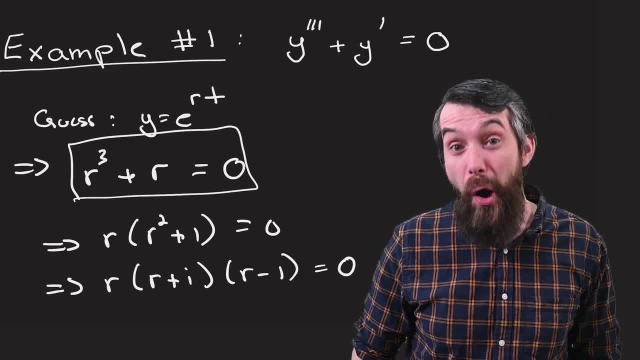 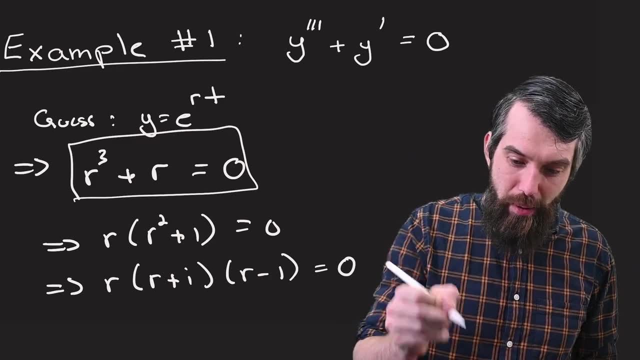 So the general methodology is to guess one solution- like we guessed the r was one of the solutions here- and factor it out, And then you're reduced down to something that hopefully you can do. Okay, so what do I have? Well, from this characteristic equation, I see now that I have 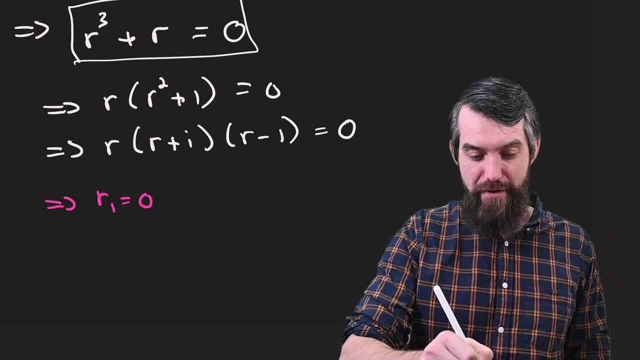 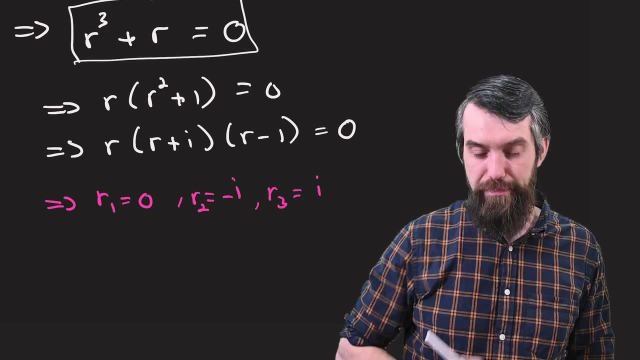 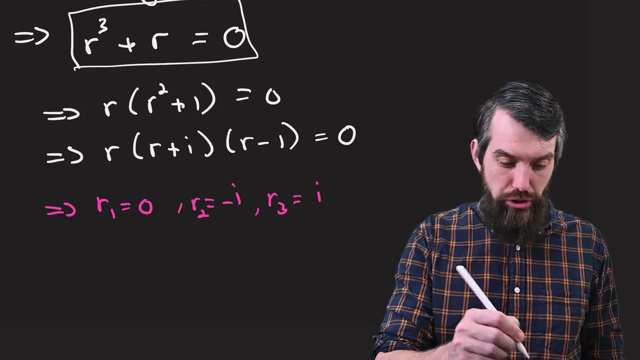 I have three different roots: r1 is equal to zero. I have r is equal to minus i, that's r2, and then r3 is equal to plus i, And then, since our solutions were of the form e to the rt, my general solution looks like this: 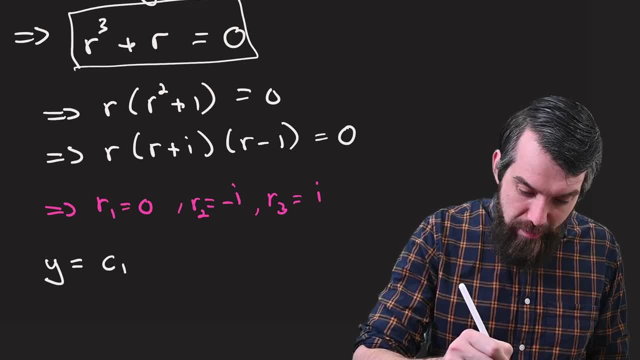 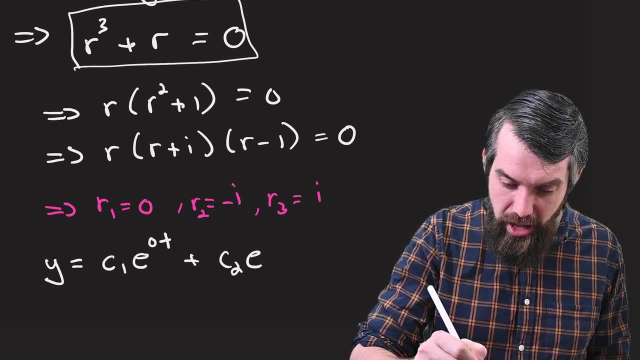 It's some generic constant: c1 multiplied by e to the Well r is zero, so zero times t. and then a constant c2, e to the Minus i times t, and then finally c3, e to the plus i times t. 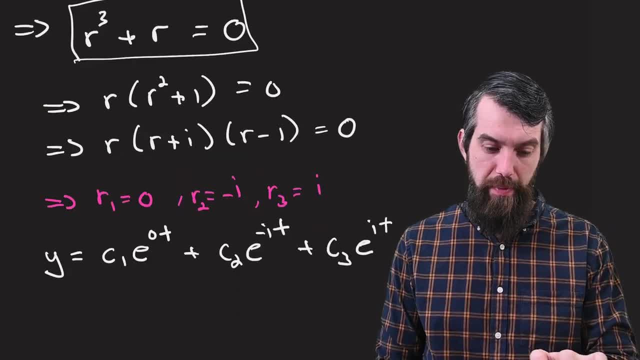 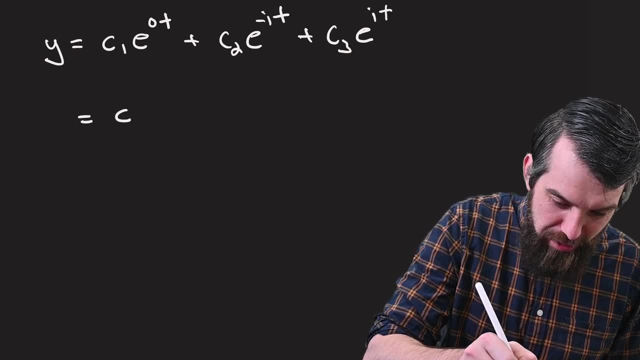 This answer is okay, but I want to do two different manipulations to it. So the first manipulation I'm going to do is: Well, I'm just going to say that e to the zero, t is just one, and so I'll just put the c1 out the front. 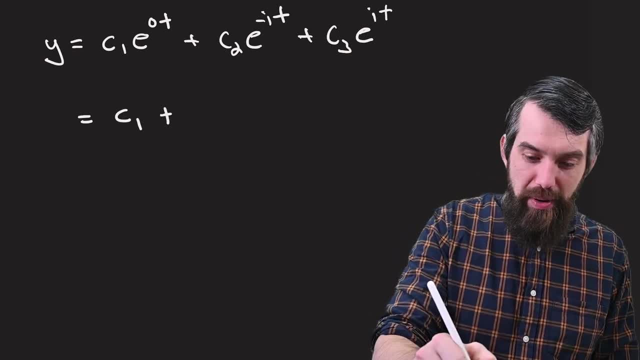 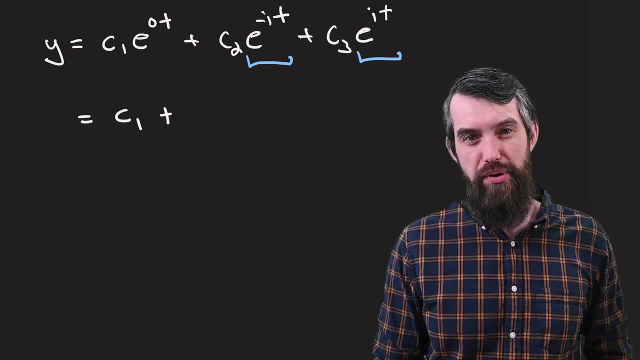 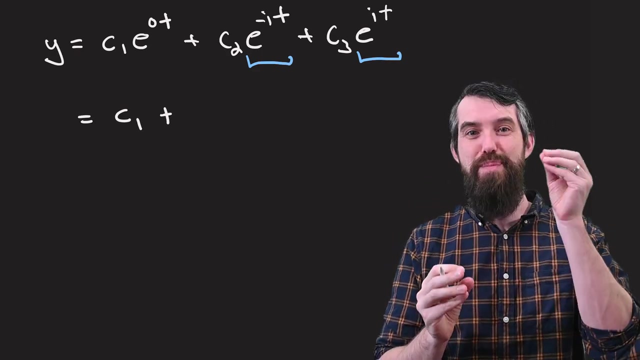 That's the easy manipulation. But then the second manipulation I want to do is I notice that I have this: two different exponentials with imaginary numbers in them: e to the minus i t And e to the plus i t. Now my goal is to take these exponentials with imaginary components. 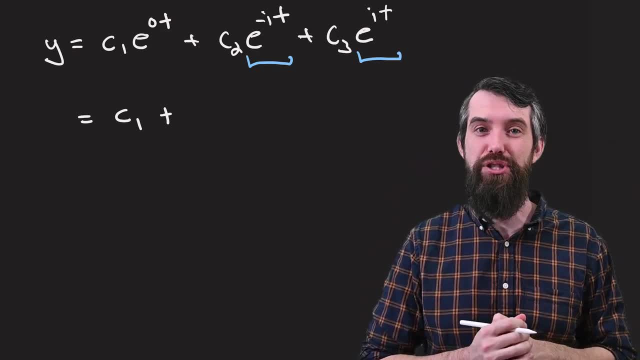 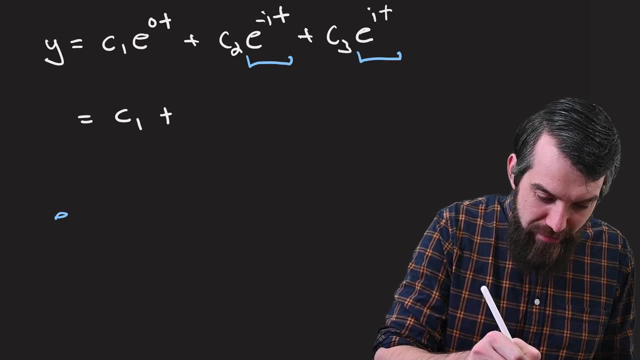 and I would like to have two real, linearly independent solutions. I can use instead The standard trick, exactly as we did when we were talking about the second order case, is that if you have e to the, say alpha plus or minus, i, beta times t, that would be the general case. 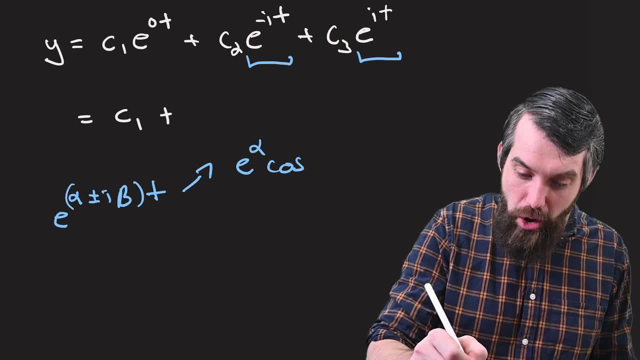 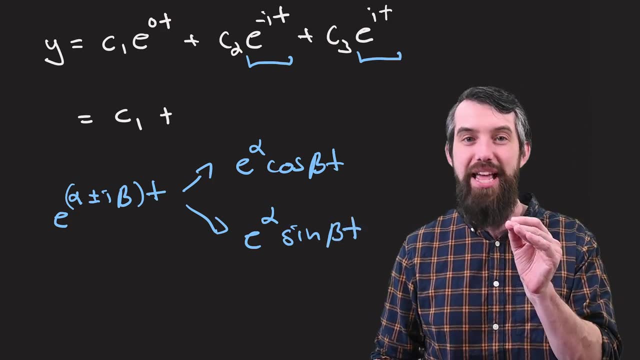 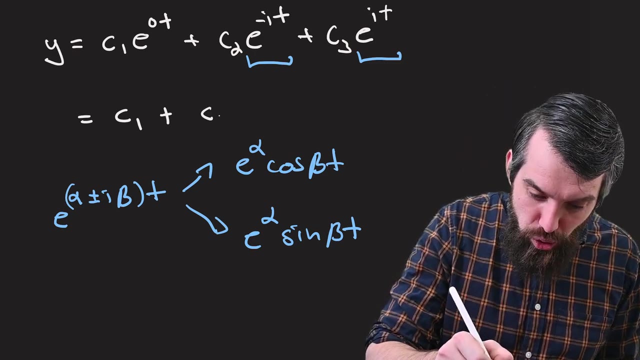 then your two different solutions are e to the alpha cosine of beta t and e to the alpha sine of beta t, And the details of that conversion we did in the previous video. So for the purpose of our example I'm just going to say c2.. 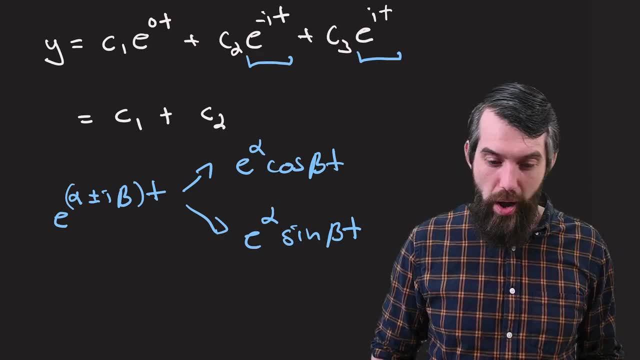 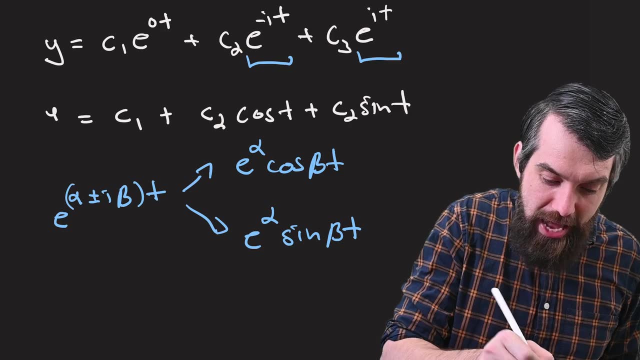 Well, my alpha is zero, there's no real component and my beta is one. so it's c2 times cosine of t plus c2 sine of t, And that is my final answer. All right, so what have we done? 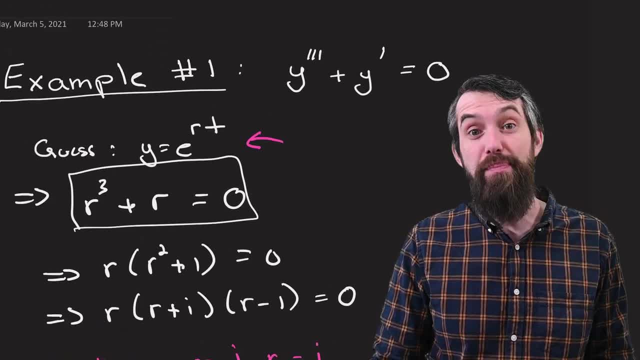 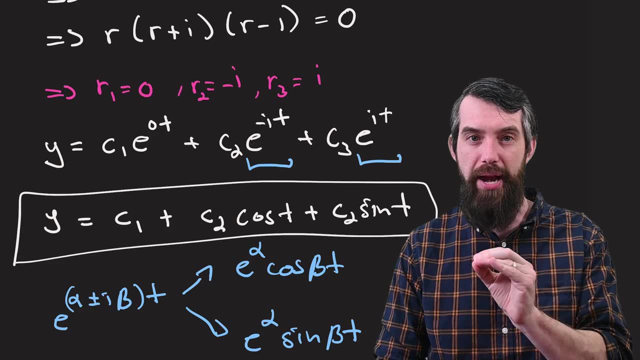 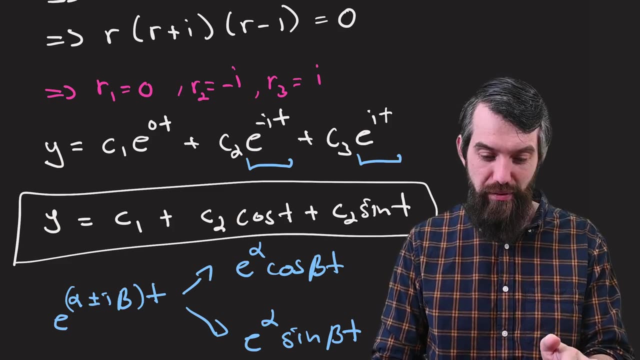 For our original differential equation, y triple prime plus y prime equal to zero, we now have this general solution: c1 plus c2 cosine and c2 sine. All right, so that was one. Let's do one more example to lock in what happens when you have multiple types of repetitions. 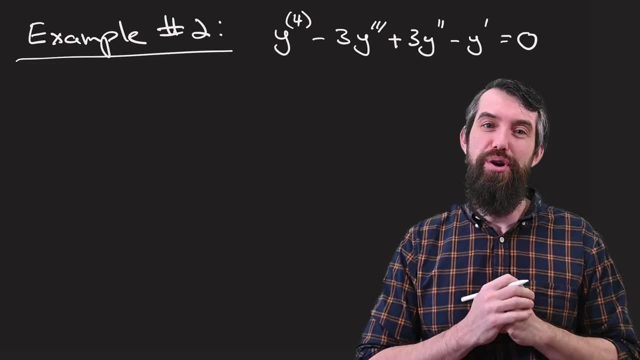 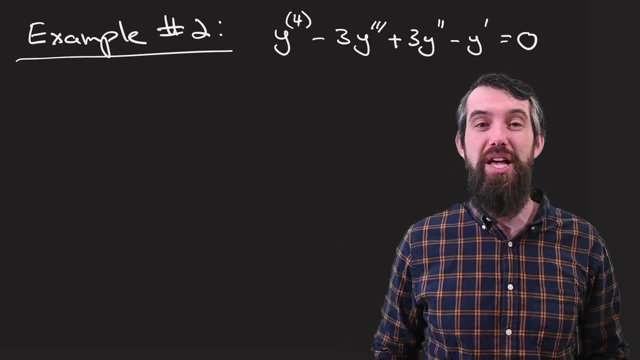 So the second example is actually a fourth order constant coefficient equation. this time It's the fourth derivative of y. When you put it in brackets you don't mean to the power of four, you mean four derivatives: The fourth derivative of y minus three times the third derivative of y plus three times the second derivative of y. 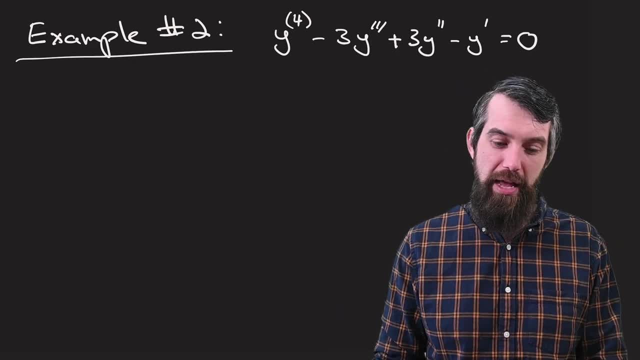 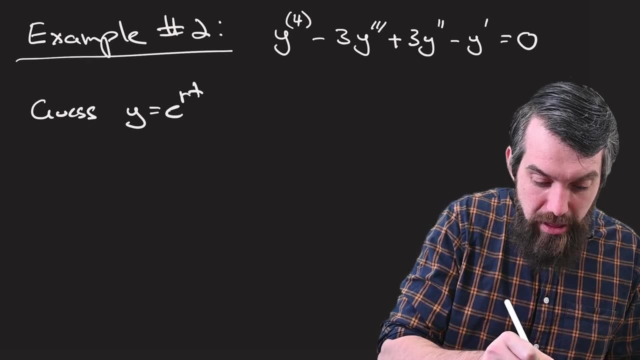 minus y, prime, all is equal to zero. Okay, a big mouthful. So we'll come up with our guess, as we always do for constant coefficients: y equals e to the rt, And this is going to give us our characteristic equation. 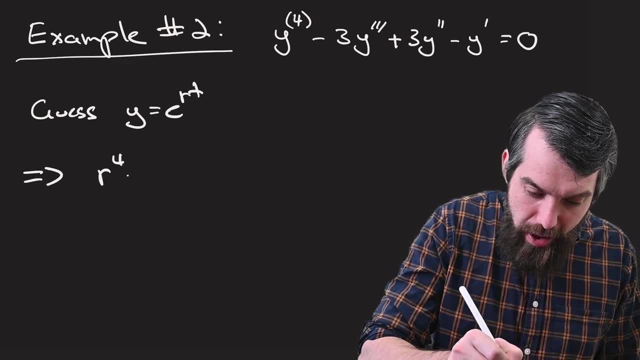 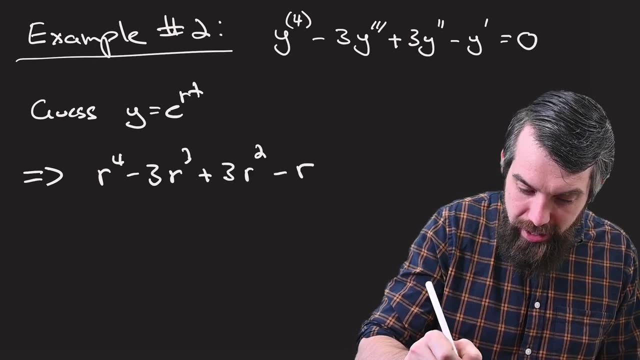 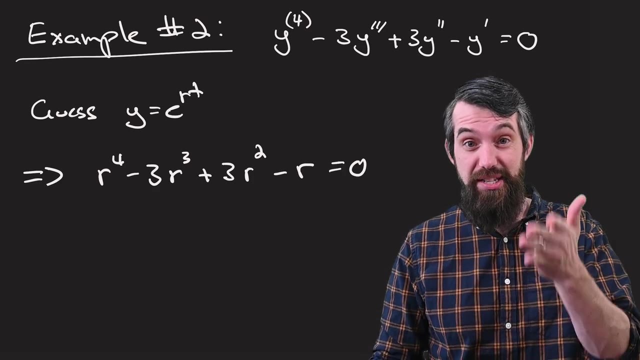 Well, four derivatives gives an r to the fourth minus three r. cubed plus three r. squared minus r is equal to zero. All of these terms would be multiplied by e to the rt. but because they're all multiplied by, So by e to the rt, I just cancel it. 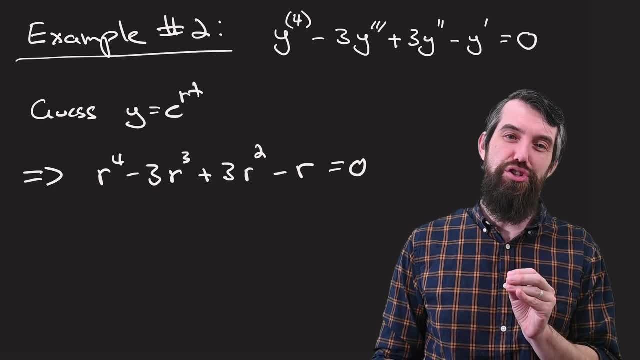 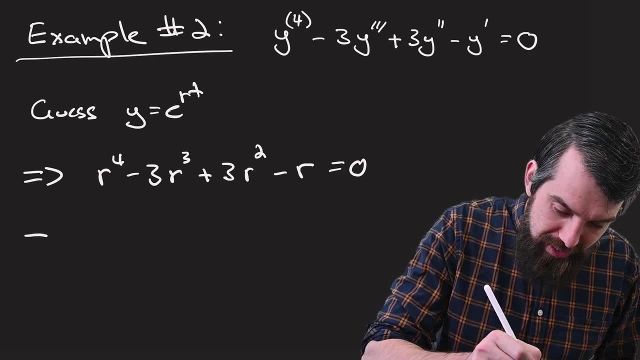 That's my characteristic equation. So now we turn to the question of trying to actually factor this. How can I do that? Well, perhaps the first thing I'll observe is that, similarly to what we had before, I see that r equal to zero is a solution. 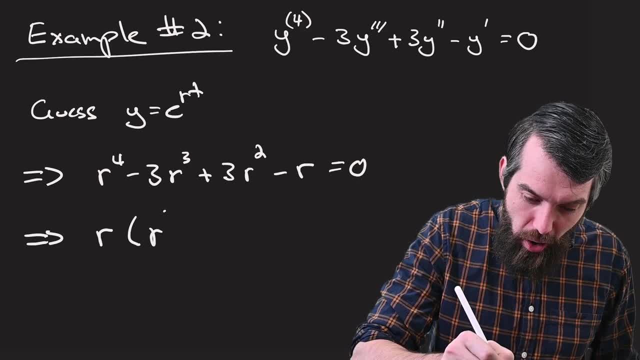 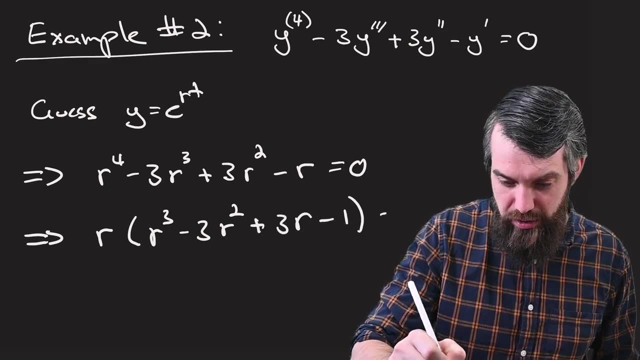 And so I can factor one r out. So that gives me r cubed minus three, r squared plus three, r minus one is equal to zero. I've made a little bit of progress. Now I have a cubic polynomial that I want to factor multiplied by r. 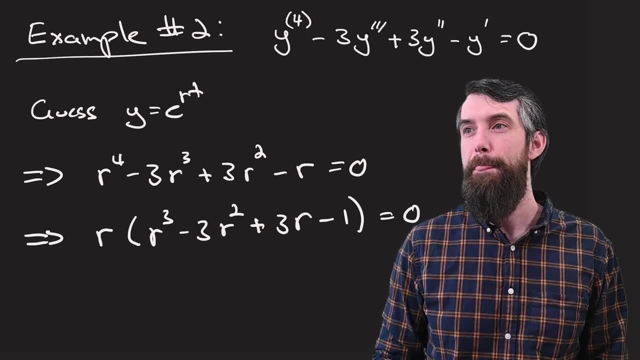 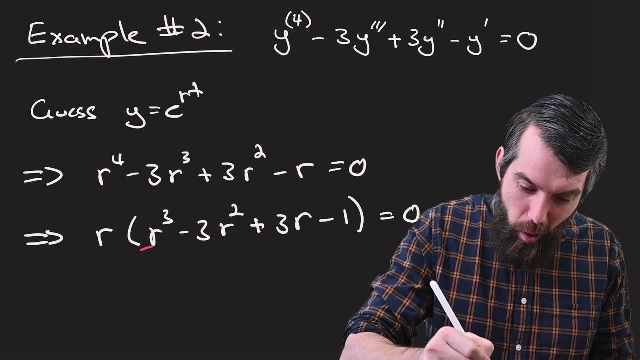 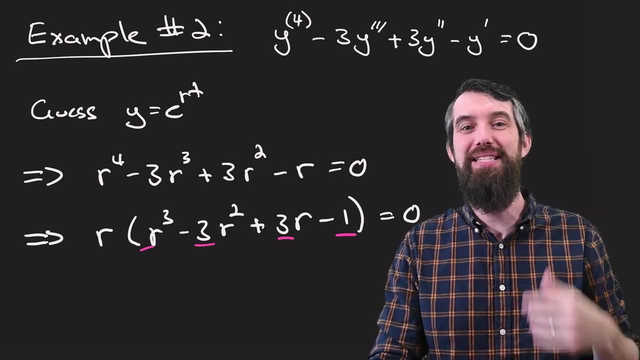 So how do I factor this cubic polynomial? Now, one thing you might just have an alarm bell going off in your head is that the numbers of one, three, three, one that looks a lot like Pascal's triangle. If you know what I'm talking about, you'll recognize that pattern. 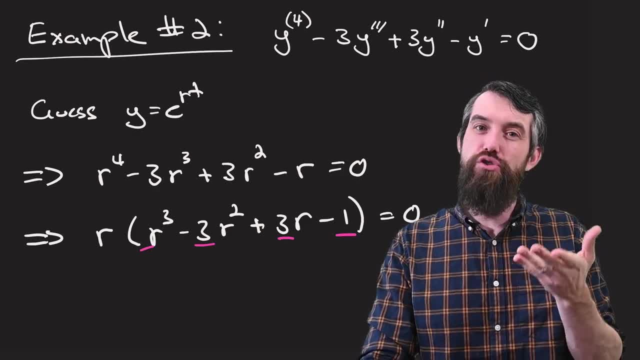 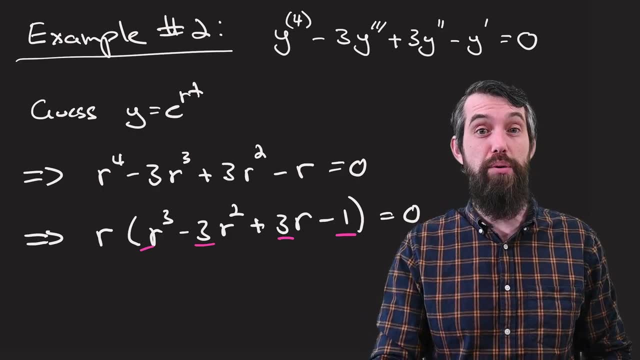 And if you don't, that's totally fine too. You can look at this and try to find one solution, And I'll just observe that if I plugged in r equal to zero, r equal to one, well, that would work. Plugging in r equal to one would give you the value of zero. 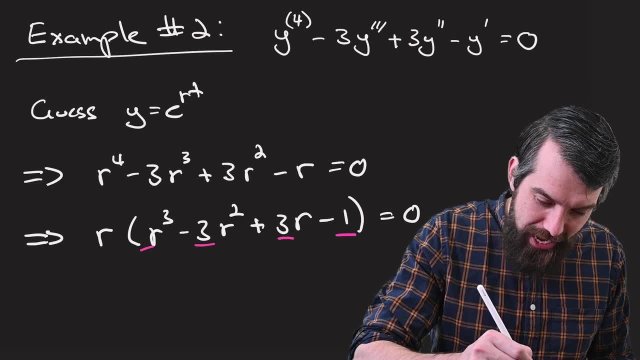 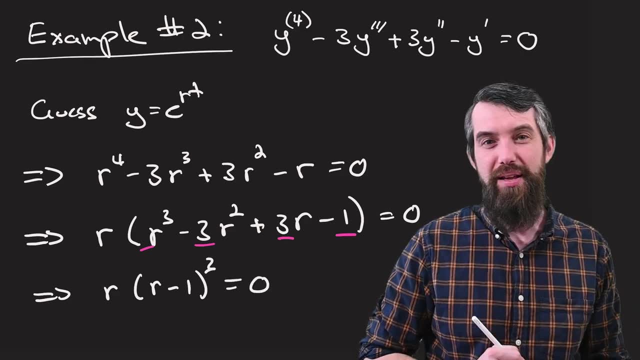 And so you could factor out r minus one, And what you actually get is the following: This is r times r minus one. cubed is equal to zero. So again, I just sort of recognize this pattern because I've seen it before with Pascal's triangle. 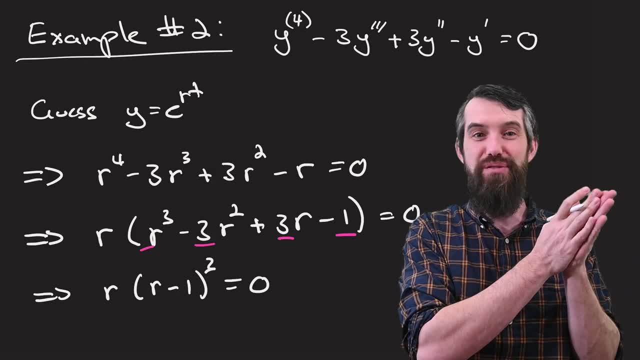 that r minus one cubed. if I wanted to expand, that would have those coefficients of the one, three, three, one, possibly with some signs, Or alternatively you have to sort of guess and find the value of r minus one cubed. 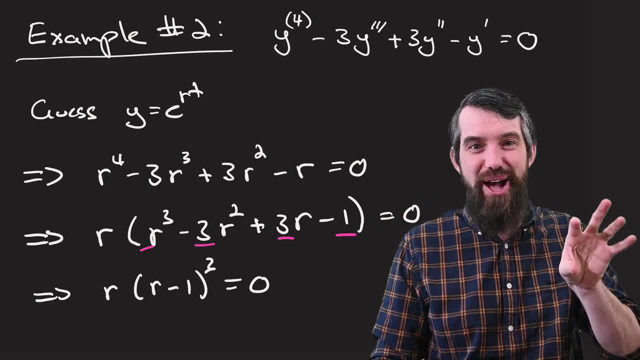 Or alternatively, you have to sort of guess and find the value of r minus one cubed. Or alternatively, you have to sort of guess and find the value of r minus one cubed, So you find that solution of r equal to one. you factor it out. 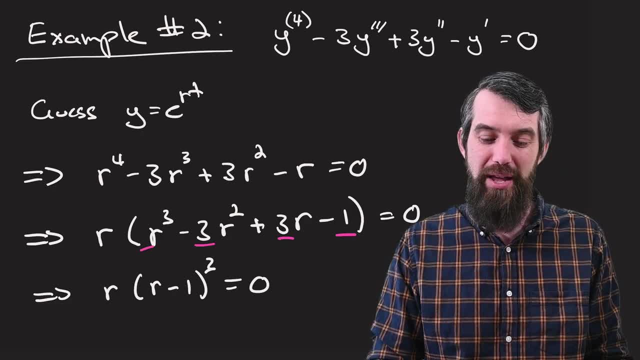 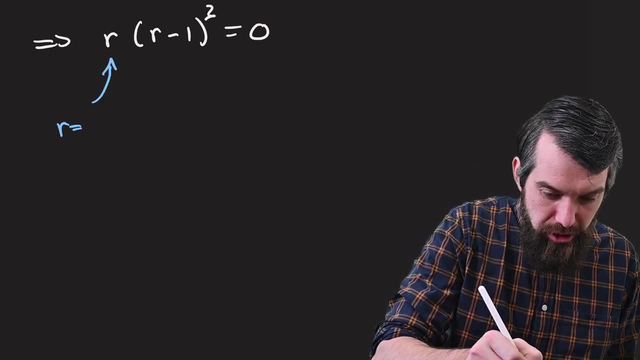 then what you'd be left with. you'd be then able to do with the quadratic formula. Regardless, I have this Okay. so now, looking at what I have, I have the following problem: I have one root here, which is r equal to zero. 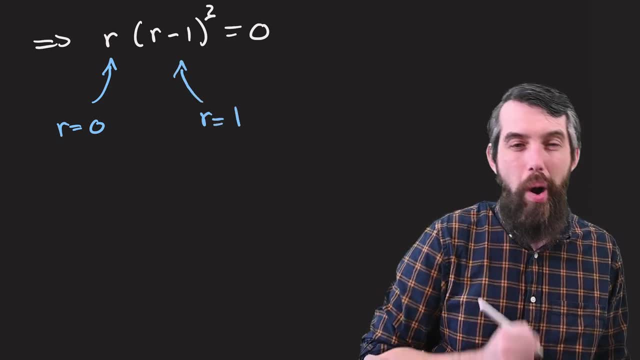 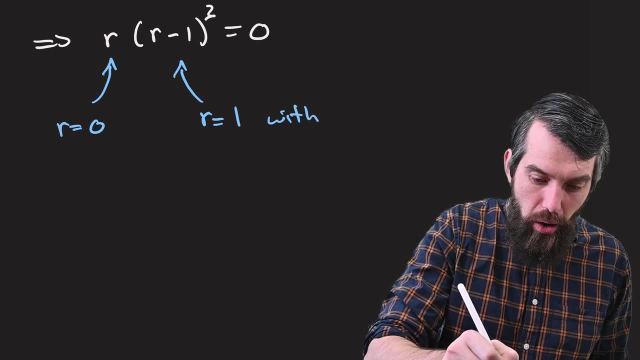 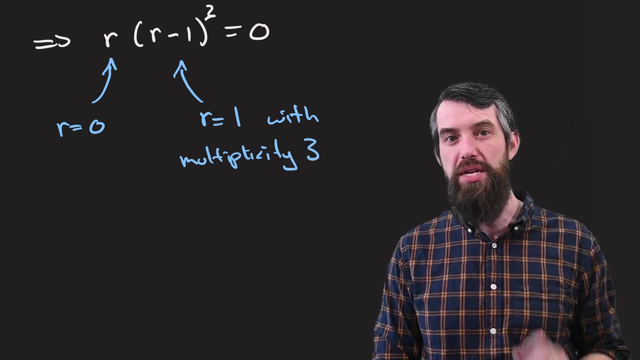 And I have a second root here, which is r equal to one. But the problem is it's r equal to one cubed. So the way I think about this is: this is, with what we call multiplicity, Or repetition, It's multiplicity 3, so it's repeated three times. 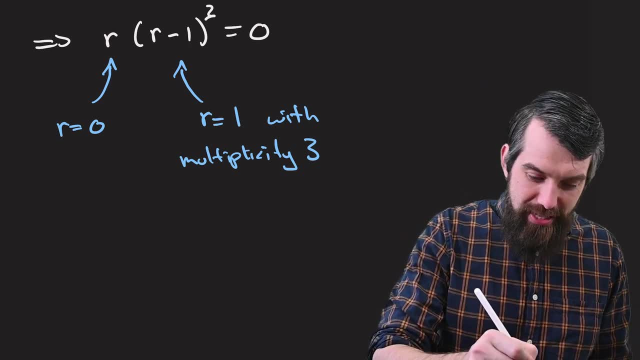 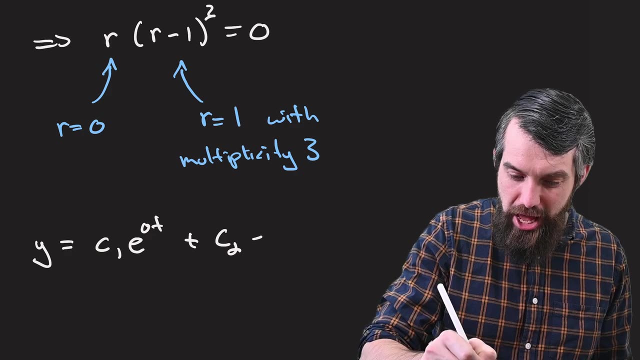 So the issue is, I can't just go and say that my solution- which I might be tempted to do- would be like c1, e to the 0t plus c2 times e to the t, that would be with r equal to 1.. 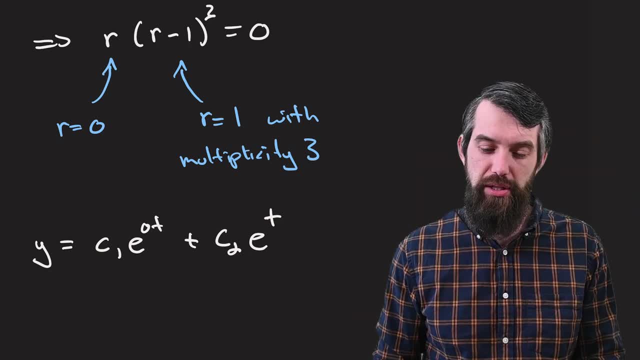 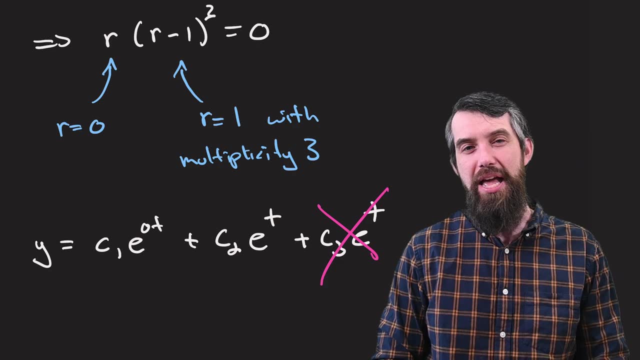 But because degree 4, and I'm looking for four literally independent solutions- I can't just go along here and say that c3 is e to the t again. This just doesn't work out. The reason is that that is just a copy of the term that I already have. 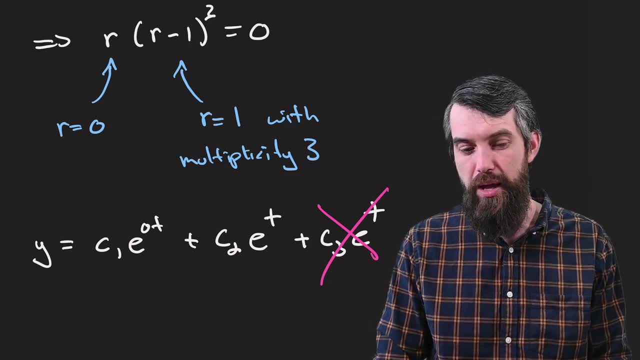 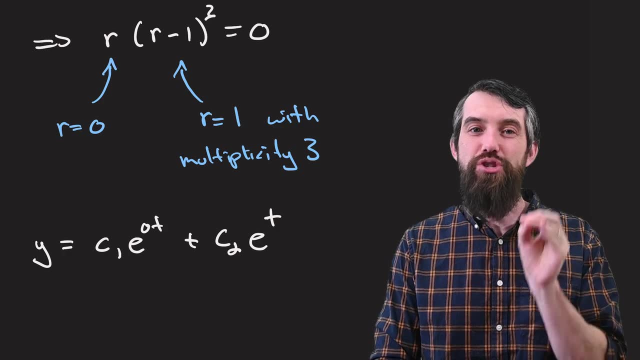 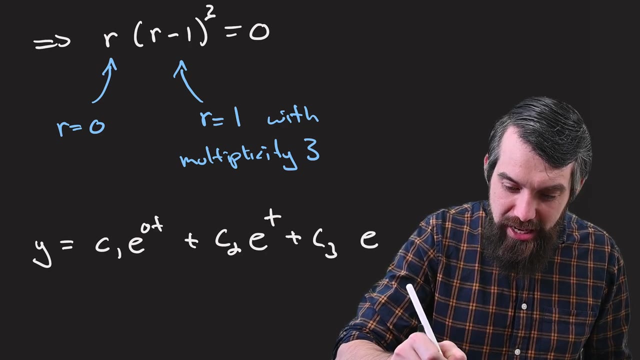 This is not a new linearly independent solution. So what can I do? Well, the methodology of repeated roots is that you can multiply by extra powers of t, and it still works out. So, for example, I'm going to take c3, and I'm going to take the e to the t, as I was anticipating. 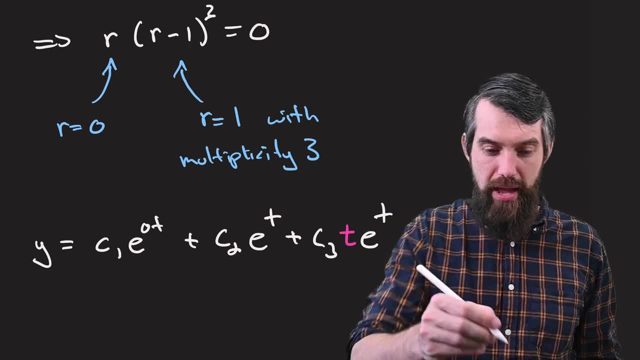 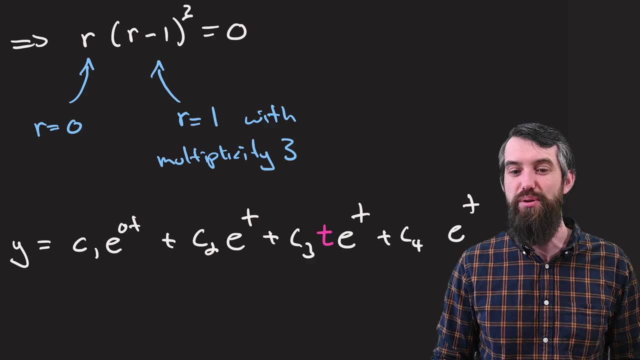 but I will make it t times e to the t, And then, in addition, I will have a c3.. c4, and an e to the t, as you'd expect, because this is the third time that the root of r equal to 1 repeats. 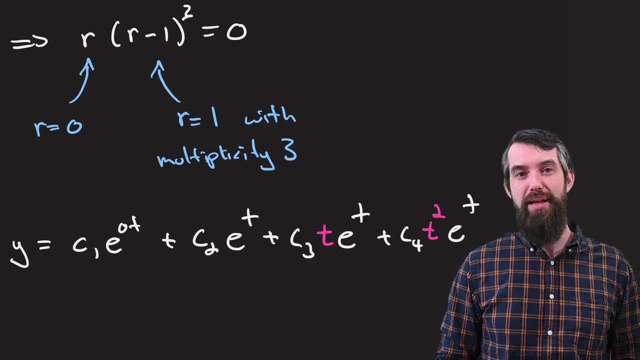 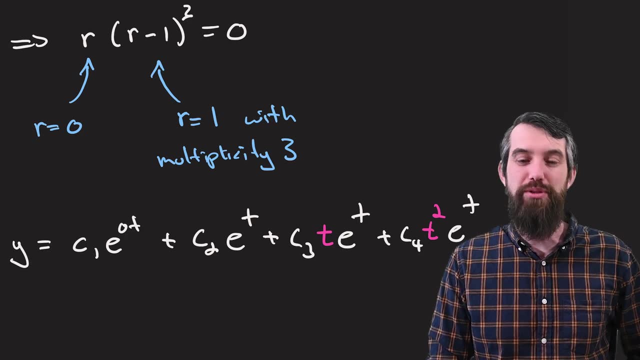 But I'm going to put a t squared in here now And in general, if it repeated 10 times, you'd be going all the way up to a t, to the 9th times, e to the t. It just depends how many times it repeats. 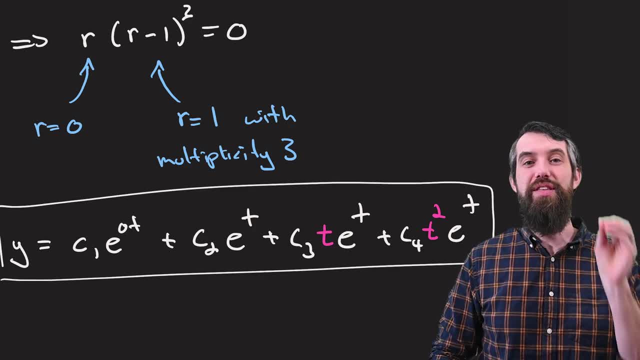 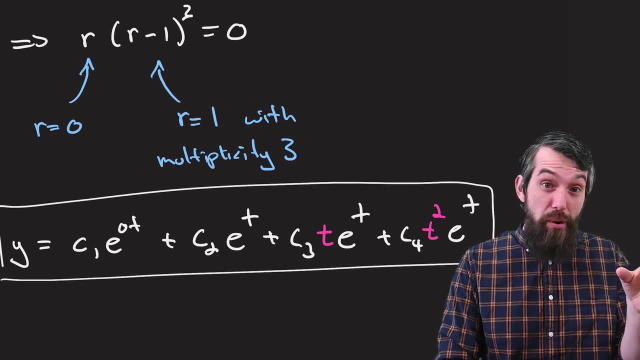 Either way, this is now my general solution when I have this repetition. So let's zoom out for a moment and try to think about how I solve all of the different ones of this category, That is, higher order, constant coefficient differential equation. Well, I'm going to plug in the e to the r t.